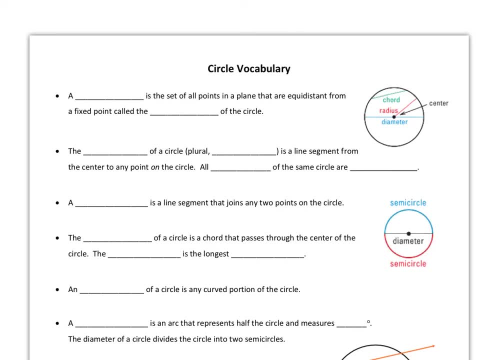 Hi guys, it's Ms Griffin. We're looking at some circle vocabulary before we dive into skill one. So you're just going to fill this out with me. You can refer back to it, kind of like you could refer back to your old vocab sheet. So we're going to start with just the 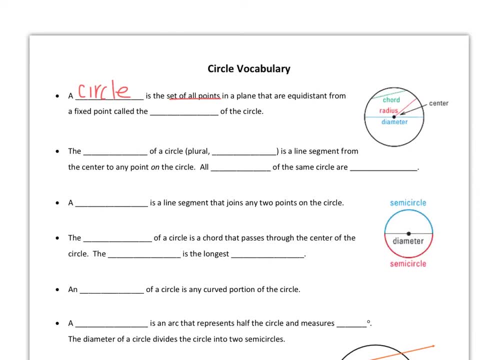 definition of a circle. It's the set of all points in a plane. so just in a space, 2D space that's equidistant from a fixed point, And that fixed point is called the center of the circle. So, if you can imagine, here's the center of the circle and every point. 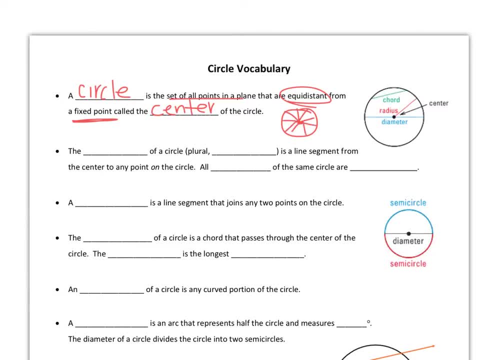 along this circle is some fixed distance. That fixed distance is called the radius, And the radius of a circle in plural form is radii. the radius is a line segment from the center to any point on the circle. So you go from the center to any point on the. 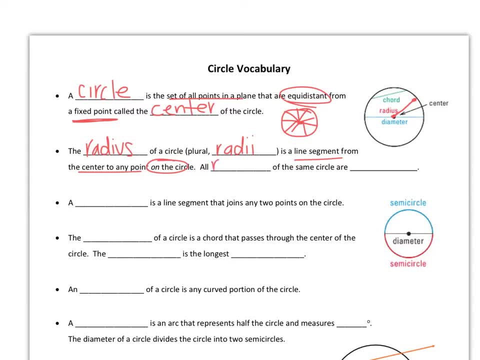 circle and you have yourself the radius. All radii are congruent within one circle Because, as I just showed you, each one of these radii are the same distance from the center to the outside on a circle, So they're all congruent to one another. The next thing we need to 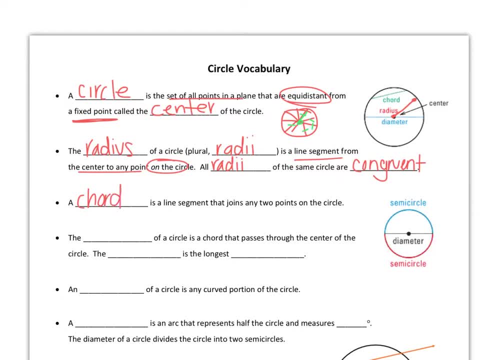 talk about is something called a chord C-H-O-R-D chord And it's a line segment that joins any two points on a circle. So if we look over here, I've got a chord connecting two points on a circle. The diameter is a super special chord Because it's a chord that passes through the center. 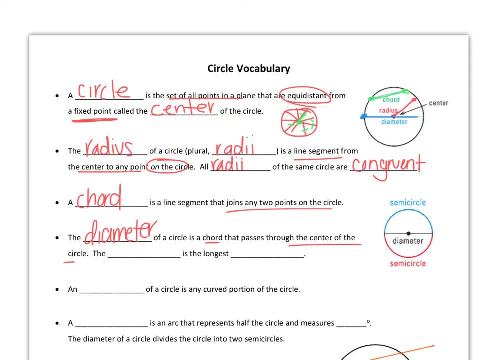 of the circle. So if we look back here at my original picture, diameter connects two points on the circle, but it passes through the center And the diameter is the longest chord. The next thing we have to talk about is something called an arc. An arc is any. 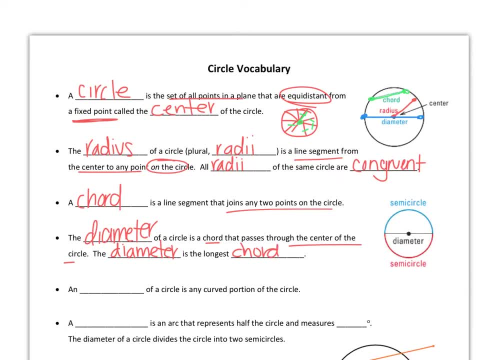 curved portion of the circle. So here's a circle with some center And I could have a point A, B and maybe C somewhere. I can talk about arc, AB as an arc And we indicate this as AB, and then you literally put an arc over it And we can talk about the measure. 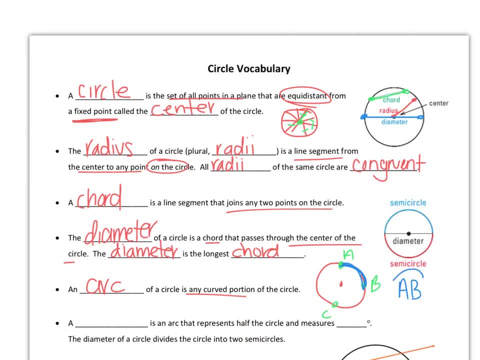 of arc AB. A book will tell you about that- And we can talk about arc Q. Here's an example- by putting the M and then the AB with the arc over it, and we can talk about it in terms of some degree measure. Those are supposed to be degree symbols. Okay, we could also. 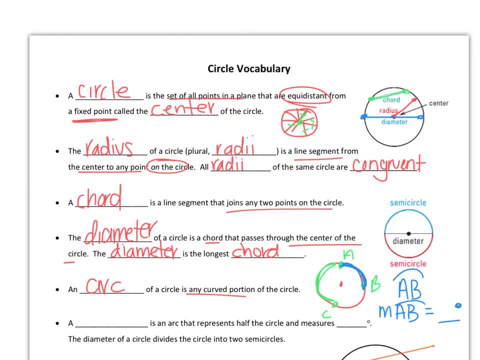 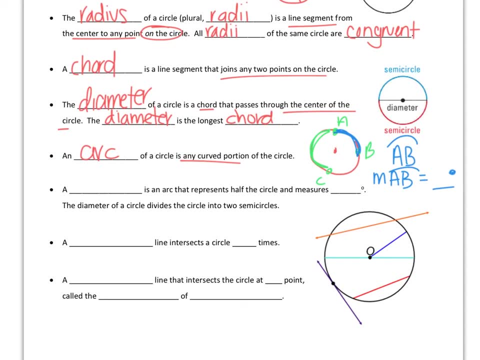 talk about arc, AC, if we wanted to, or BC, etc. etc. The next thing we want to talk about is something called a semicircle, And a semicircle is an arc that represents half the circle. So if you think of a full circle, you should write this down somewhere: full circle, the 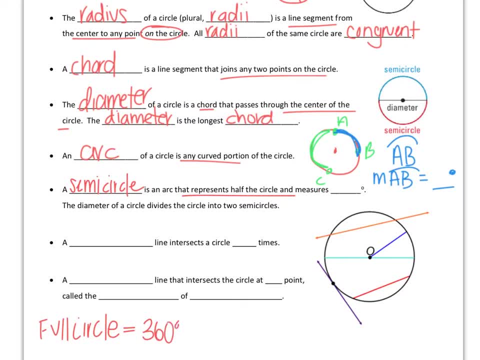 arcs equal 360 degrees. So a half of a circle is half that 180 degrees. The diameter is what divides the circle into the two semicircles. So here's a picture to indicate that Diameter cuts a full circle in half, into this red half and into the blue half, to make two semicircles. 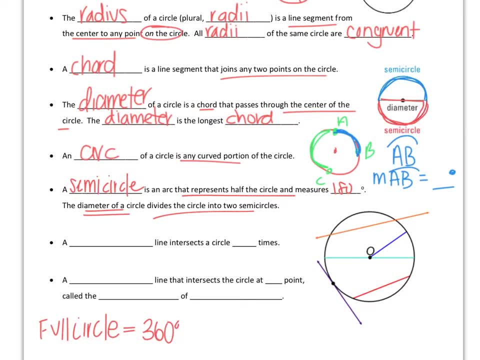 Now we're going to talk about some more segments within circles. So we've got something called a secant line- S-E-C-A-N-T- secant- And it intersects a circle two times. So this orange line right here crosses through the circle, So it doesn't stop inside the circle, it goes. 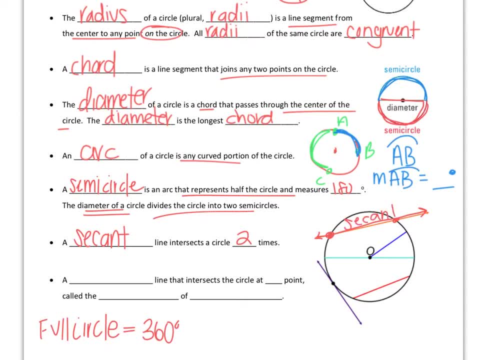 beyond it. That's called a secant, Then our next one is called a tangent. So we're going to talk about a tangent line. You've heard that word before in trig. A tangent is a line that intersects the circle at one point and only one point. So this line here hits the 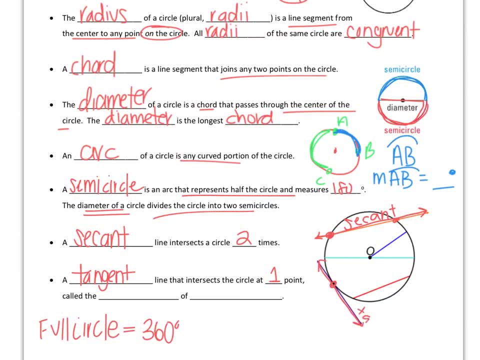 circle one time. so this is called the tangent line And that point has a super special name. It's called the point of tangency, And I'm just going to kind of draw that arrow over here. Point of tangency. There's a couple. 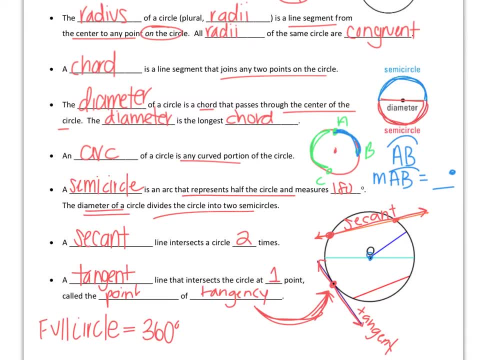 other pieces on this circle that we want to label up. So the thing that goes from the center to the outside should be non-issue for you at this point. It's called a radius, The segment that goes all the way across through the center, connecting two points on the circle. 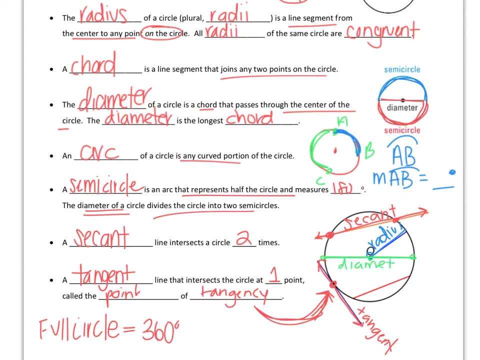 is called a diameter, And then the piece of information that just connects two points on the circle doesn't pass through anything special is called a chord. Okay, now that we've got the vocab down, we're going to flip over to the next page. You'll 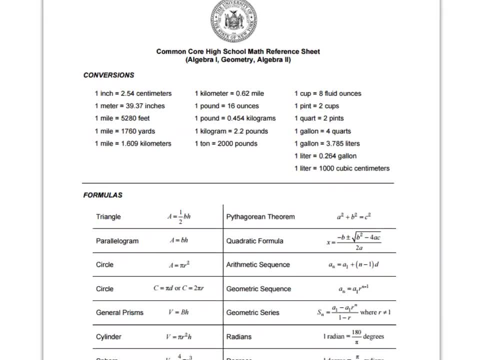 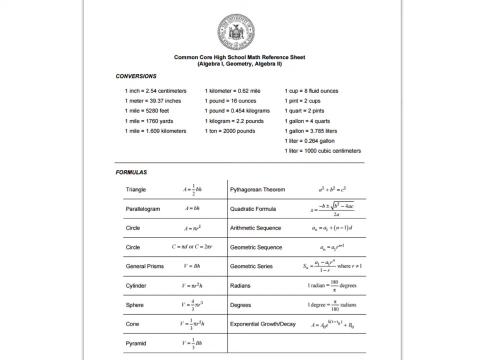 notice your reference sheet here. You probably won't be using it a whole lot in this unit, but it's there in case you need it. So let's flip to the next page to actually start skill one. All right, So here we go with unit ten, skill one A, where we're asked to find central angles and inscribed 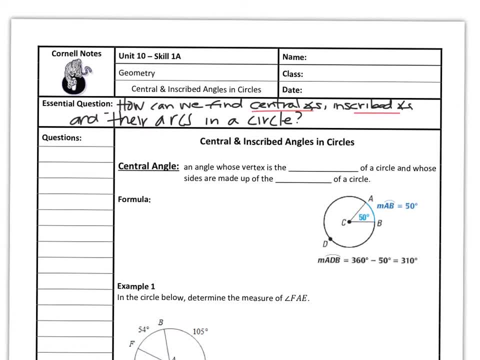 angles. So here's your essential question: How can we find central and inscribed angles and their arcs in a circle? So there's two different angles we're going to focus on today. One of them is called a central angle, the other one is called inscribed And, if you can imagine, a central angle is. 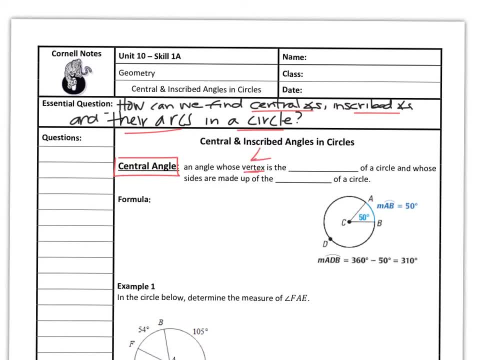 named a central angle because the vertex, so that like little corner part of an angle- is the center of a circle. Okay, the sides of that angle, so here and here, are made up of the radii of a circle. We've got a 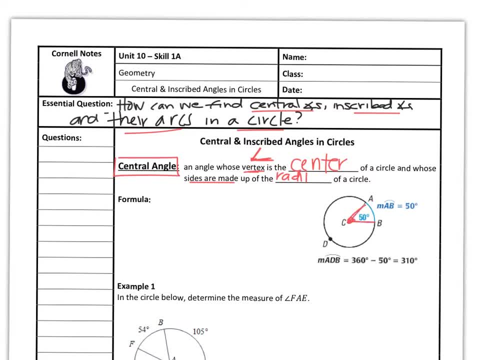 central angle here, formed at center C. The sides of that angle are made up of radii and of course those are congruent. but we don't need to mark that up because that's not the important, crucial thing here. So a formula that you have to memorize, and it's hardly a formula at all, because it's like: 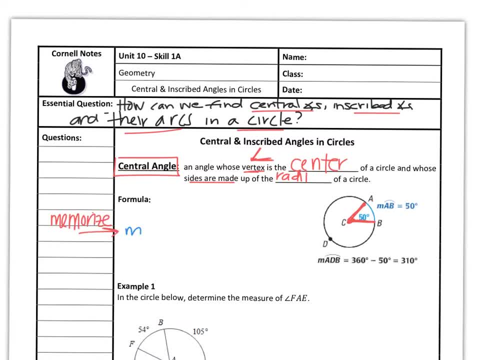 super easy is that the measure of a central angle equals the measure of its arc. Okay, so I just want to remind you that measure, and then parentheses, or the M in parentheses means measure up, All right. so when I look at this picture, we've got angle ACB is 50 degrees, and when I follow, 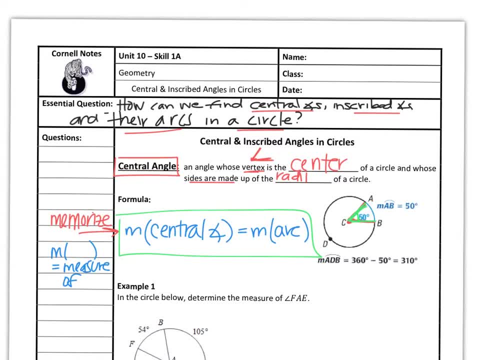 the sides of the angle out. you're going to get in the habit of doing that constantly. Follow the sides out And you'll see that it opens up to arc AB. So if the angle is 50,, therefore the arc is 50.. 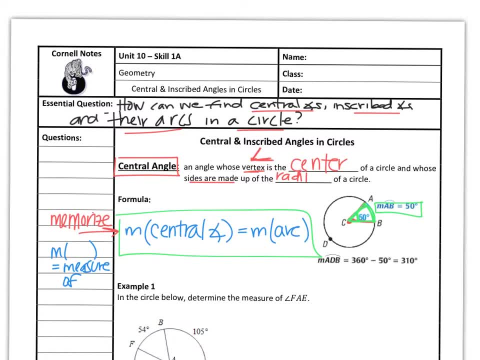 Okay, that's going to be important to remember. Central angle equals arc. Another thing that I want to point out to you is that I could find the measure of arc ADB now that I know that arc AB is 50. So ADB, the arc is just a circle's total, arc 360, take away 50 to get me 310. So this arc out. 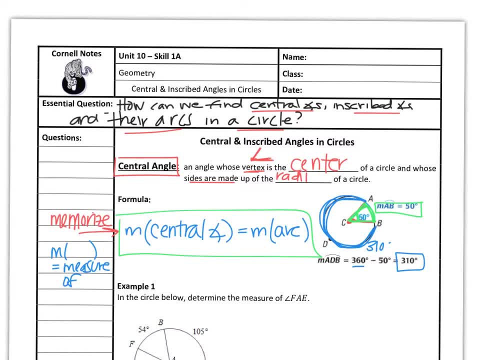 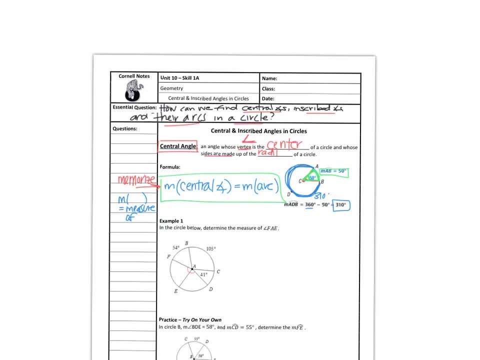 here is 310 degrees. Okay, you didn't need to know that right now, But it is something that's easy enough to just talk about real quick. There's going to be a couple pieces of information for each of these examples that is helpful to. 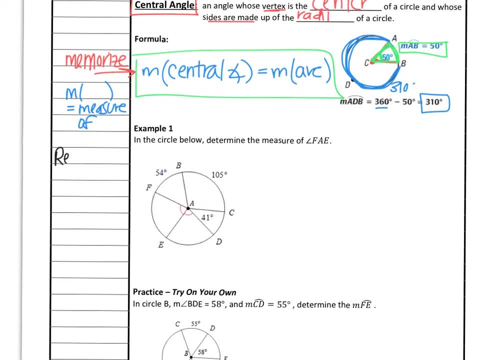 recall, So I want to write some recall pieces over here. Recall first off the angles on a line equal 180 degrees. Secondly, you should remember that vertical angles are congruent and those are the ones that are in an x and across from each other. You also need to: 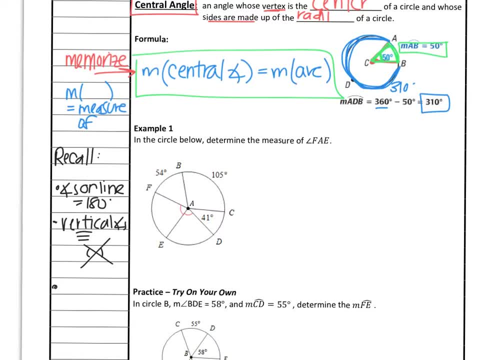 remember that we just talked about it, that angles in a circle equal 360 degrees And same thing with arcs in a circle. Okay, so when we look at this first example, it says: determine the measure of angle f8,, e, f, a. 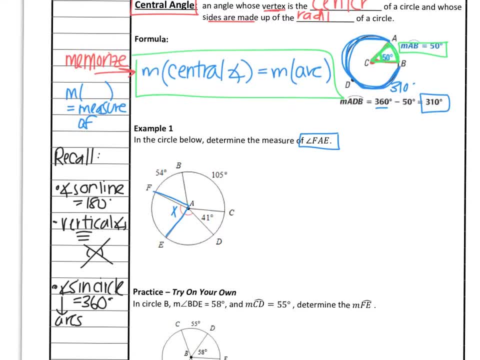 e. So that's this one. But I also notice that this angle is marked congruent to this angle. So if I called FAE as X, then I'm going to call this one as X And I notice that angle. FAE opens up to arc FE, kind of like slicing a pizza. 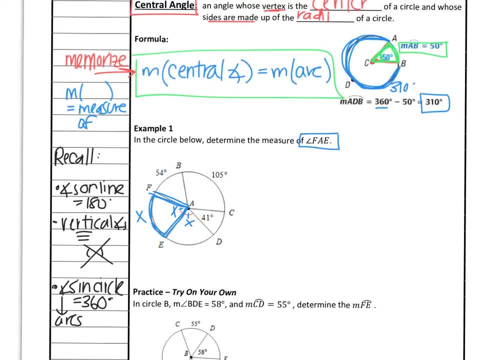 And this is my crust. The crust has an arc measure of X, And so would this one, because here's my pizza slice. I open up and I have arc DE and here's X. This angle, FAB, opens up to arc FB, and that arc is 54, therefore the central angle is also 54.. 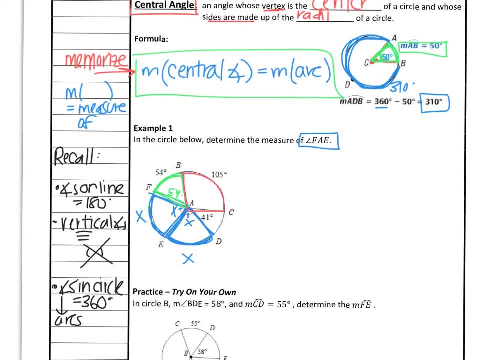 Assuming you could guess what angle BAC would be. the central angle is opening up to arc BC, and so its measure is 41.. And, last but not least, we've got this one. You want to just fill in as much information as you possibly can using this piece of given information. 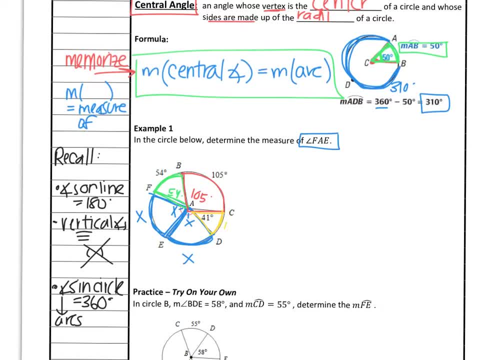 Angle CAD is 41,, therefore the arc is 41. So I can think about answering this question in one of two ways. I've got a full circle's arcs all labeled up and a full circle's arcs equal out to 360.. 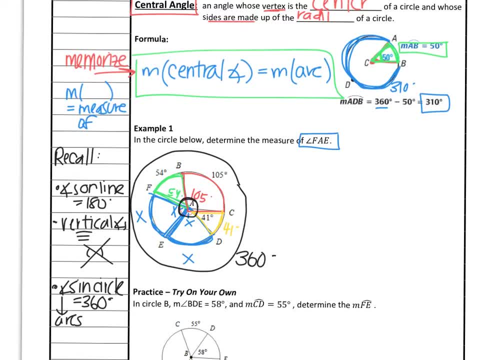 Or I have a full circle's angles on the inside that equal out to 360.. So either way you're going to be fine. I've got an X and an X. so 2X plus 54.. Plus 105, plus 41, equals 360.. 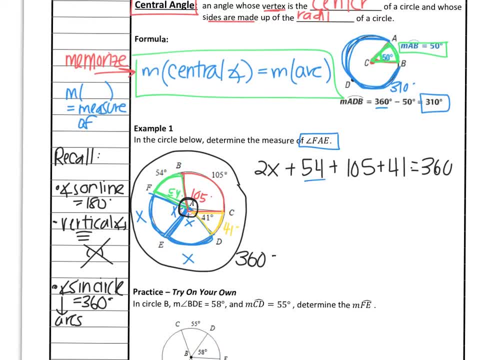 Alright, so, doing a little bit of math, we're going to keep the 2X, but I'm going to add these three pieces. So we have 2X. these three pieces sum to 200, and that's equal to 360. 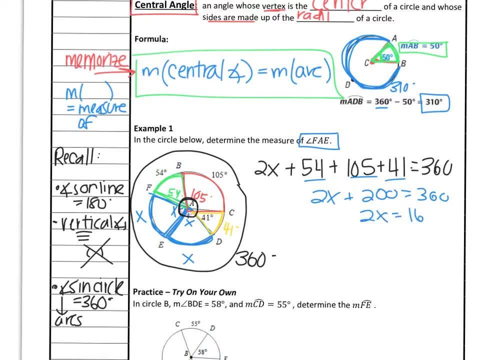 Then I subtract away the 200, so I have 2X equals 160, divide by 2, and X equals 80. And remember that I did call my original piece of information that I needed as X. So I'm going to say the measure of angle: FAE equals 80 degrees. 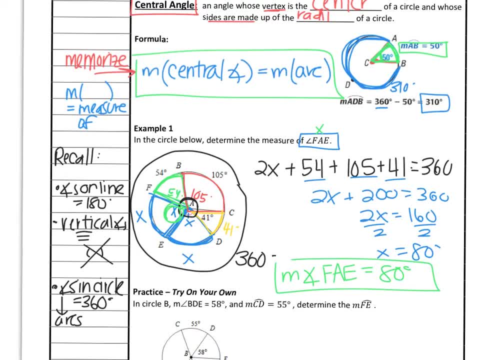 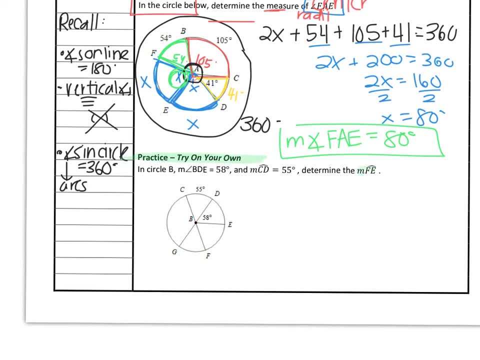 And that one's done. The next one is for you to try on your own. So you're going to give this a whirl, try it on your own right now, And then you're trying to find the measure of arc FE. so that's this piece of information right here. 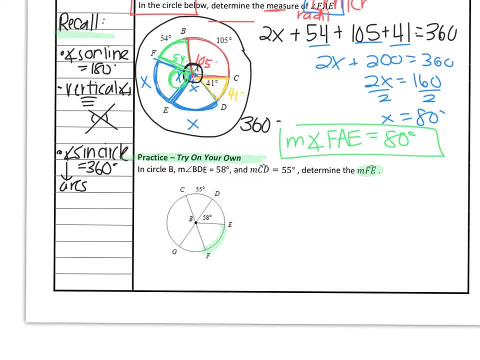 Alright, and don't forget to recall this information: Angles on a line, vertical angles on a line, Angles, angles in a circle and arcs in a circle. Give it a try and then I'll put the answers up so that we can talk about it together. 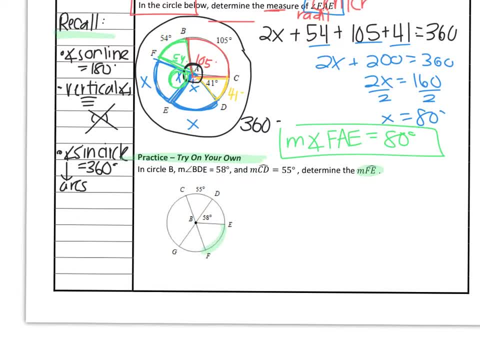 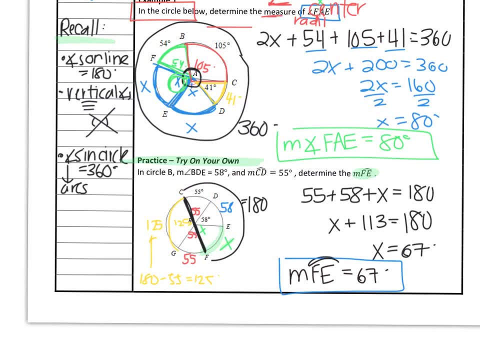 Pause the video while you do it. Alright, so you can see my work written down here. First I found out each arc and each angle just by using the formula that the angle equals the arc that it opens up to, And then I noticed that I had a big diameter here. 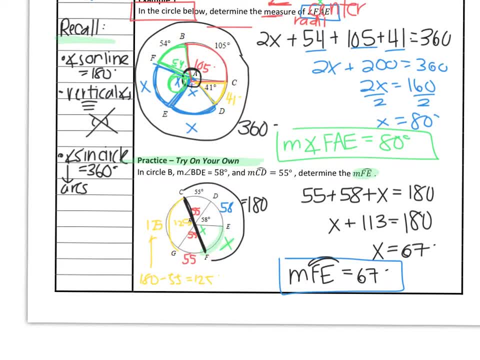 And so I chose to look at the arcs on a semicircle adding up to 180.. You could look at the angles on a line Adding up to 180.. And so I just made a quick equation and solved it for x. So the measure of FE is 67.. 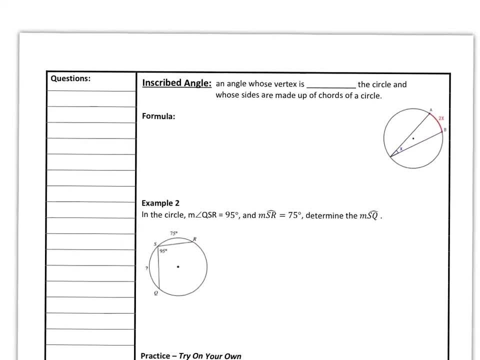 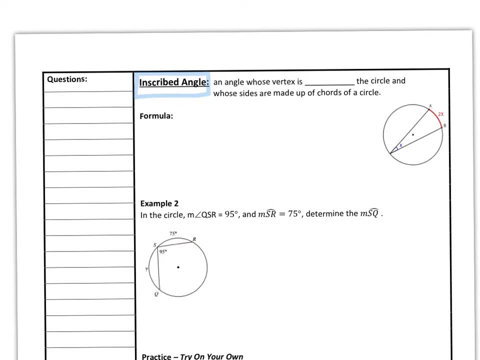 On this page, we're going to be taking a look at something called an inscribed angle, And so this is the second type of angle that we're talking about today, That you do have to memorize a little bit of a formula for, but again, it's not hard. 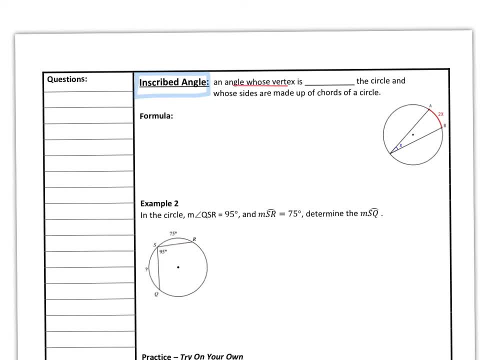 Inscribed angle is a vertex or an angle whose vertex? so that again pointy part is on the circle, So not at the center but on the edge of the circle. Here it is right there, And the sides are made up of chords. 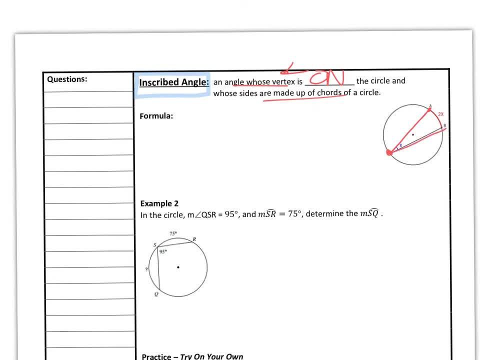 So, remember, a chord connects one point to another on a circle. So an inscribed angle is like a I don't know a really long angle, sometimes, Depending on how those chords are situated, But it's always on the circle itself And our formula here says the measure of an inscribed angle is equal to the measure of the arc. 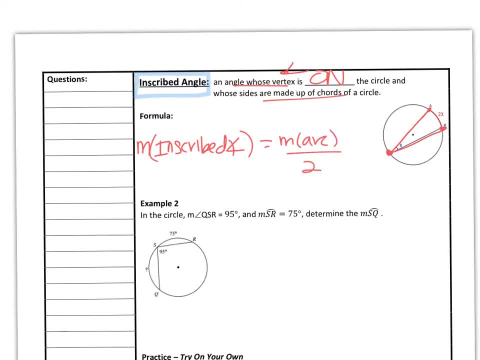 Divided by 2. And if you want, you can put this over 1 so you can cross multiply if necessary. But there's a quick trick to this and it's really actually quite easy If you start at the angle and you go outwards. 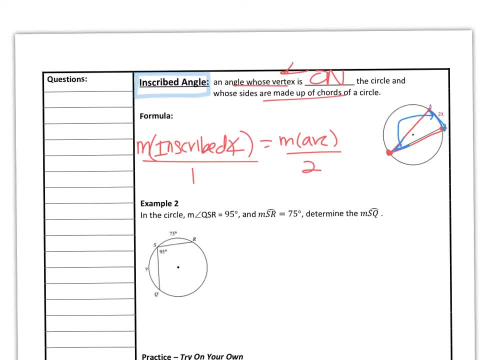 Notice how the angle is very skinny here and the arc is quite large in comparison. We have to multiply by 2 to find the arc. If we start with the arc and we go inwards, we're getting smaller. so we just simply divide by 2.. 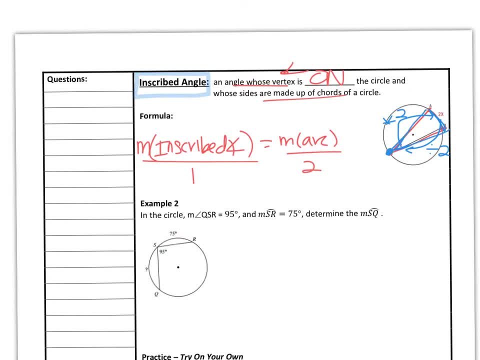 It's only if the angle is on the edge of the circle. Okay, so going out is multiply, going in is divide. So we're going to apply that in example 2. here It says we've got angle. QSR is 95 degrees. 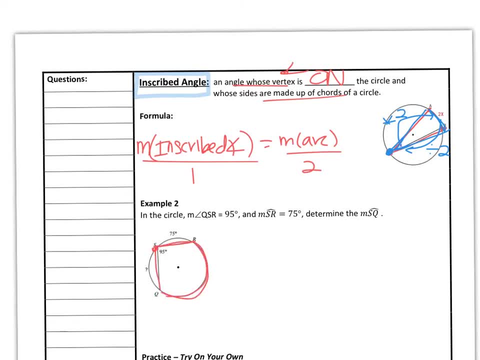 And notice that this is on the edge of the circle and so it opens up to arc QR. Arc SR is 75, determine the measure of arc SQ. So I'm going to put an X over here where SQ is, I'm going to highlight that in green and I'll highlight the other arc in blue. 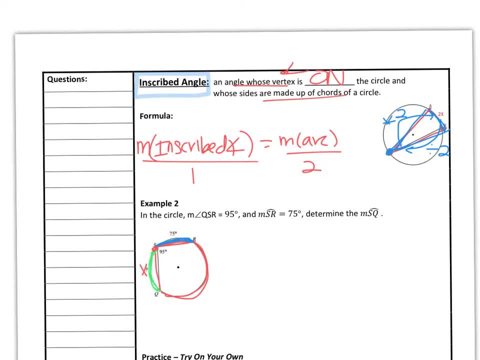 Just so I can see the three of them. So again I notice that this inscribed angle opens up to this arc. here We've got another pizza but we're cutting it. really weird. I've got to go outwards to find that arc. 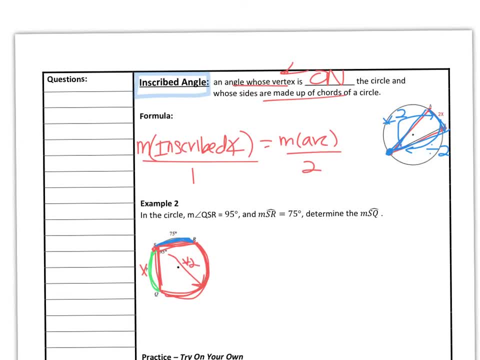 So I'm going out, which means I'm going to multiply by 2.. So 95 times 2. And that gives me 190.. From there I'm going to label it and that's my arc from Q to R. And then I notice that my arc from Q to R is 90 degrees. 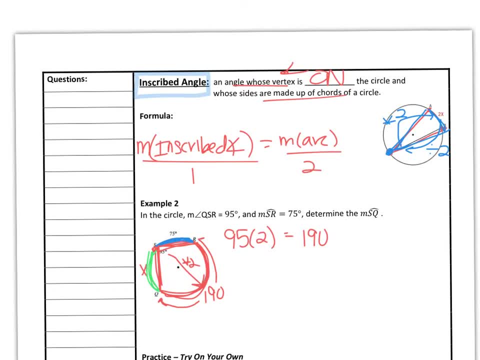 So my green, blue and red arc all make a full circle. So we've got a full circle with X, 75, and 190. And a full circle means we're going to add up to 360.. So step one was find the outside arc. 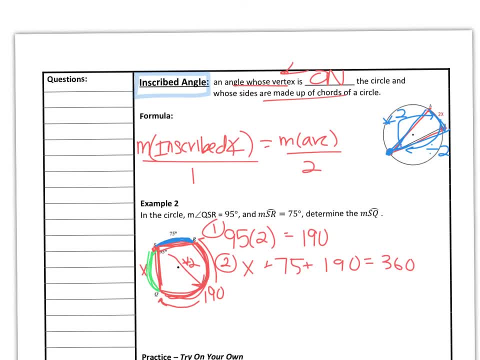 Step two is now find the missing piece of information by adding the 360.. So I have these two numbers which can combine: X plus 265 equals 360.. Subtract and we get X equals 95 degrees, So the measure of arc SQ equals 95.. 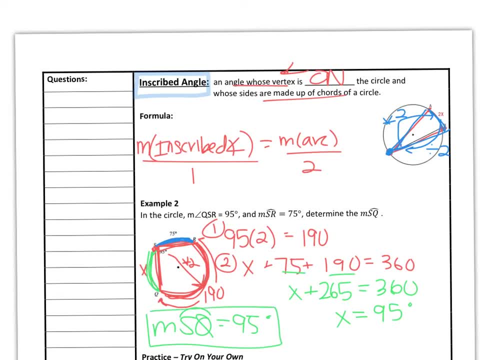 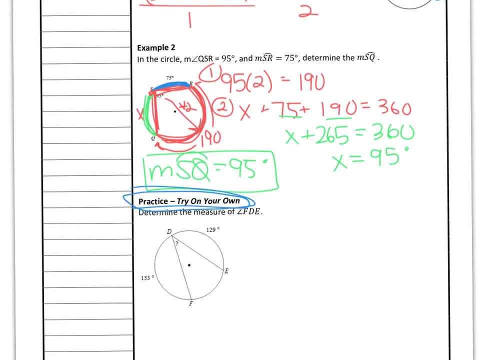 And no, it's not because there was already a 95 on the picture, It's just a coincidence. Okay, so here's a practice problem for you to try on your own And again, actually try it first. Your goal is to find the measure of angle FDE. 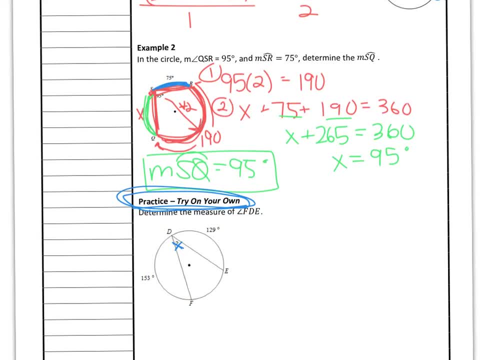 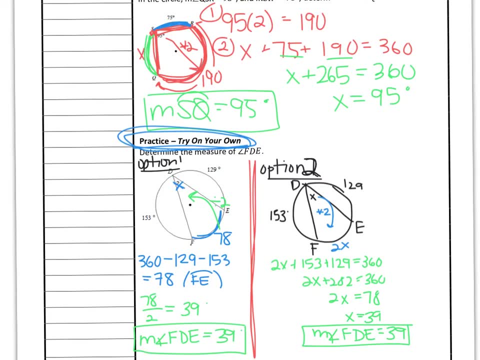 So I'm going to place an X here And then you're off to the races solving for X. All right, so I did this in two different ways, just in case you did it in a different way than I did. So option one is to find out this missing arc first. 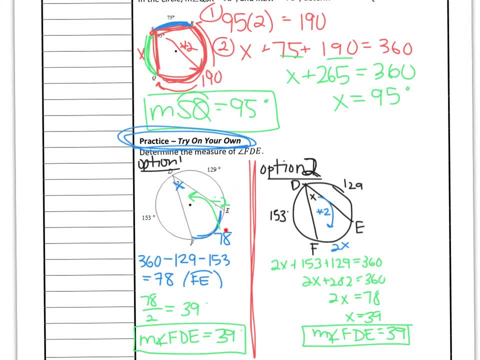 So I know that the three arcs here make 360.. I subtract away from 360, and I find arc FE has the measure of 78. So I plop it here. And then I know that to go inwards to this angle I have to divide by 2.. 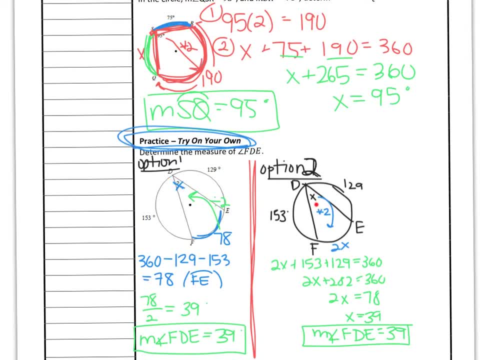 So 39 is your answer. The second option is to take your X, multiply it by 2, because you're going outwards from an inscribed angle. Going out, multiplying by 2 gives this arc a measure of 2X right now. 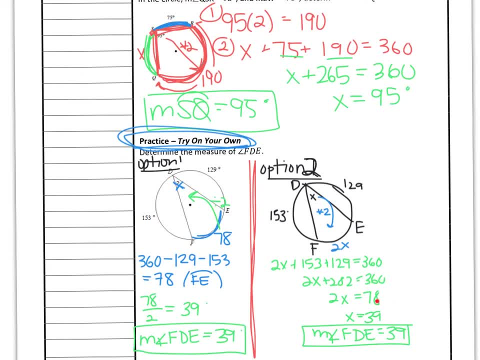 And then, I know, all three of them add up to 360.. I divide, I subtract, et cetera, et cetera, and I get 39. So either option is totally fine. You see that we get the same answer in both places. 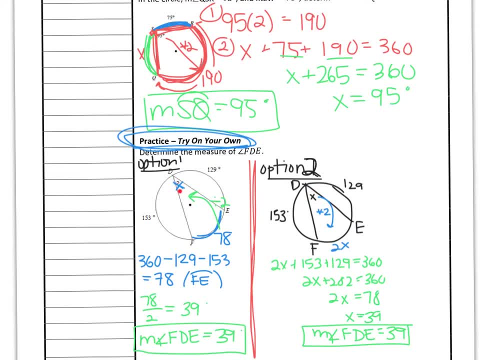 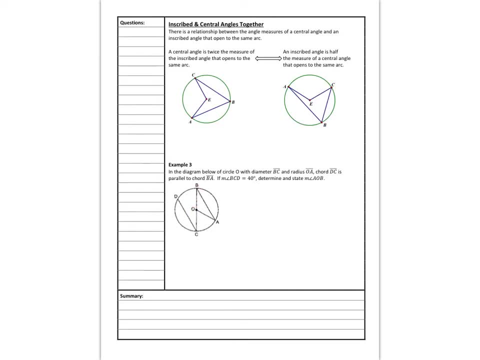 As long as you call this initial angle as X, then you're good to go Flip it over. We're going to see a combination of the two things together. So if we're talking about this, if we're talking about inscribed and central angles together, 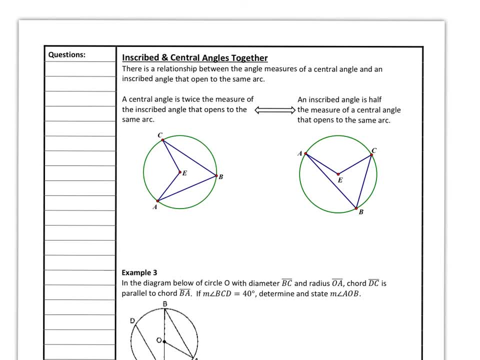 there's this relationship because if they open up to the same arc, then there's something super special. So notice how this central angle opens up to arc AC and this inscribed angle opens up to arc AC. So if they both open up to the same arc, 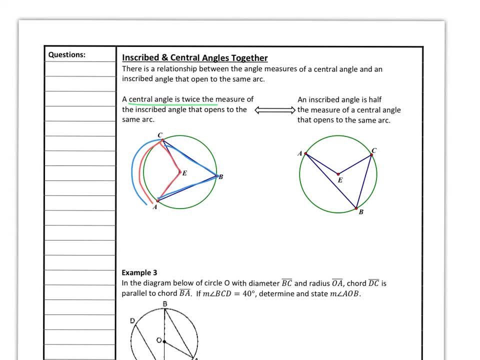 then there's this relationship that can be written in one of two ways: The central angle is twice the measure of the inscribed angle When they open to the same arc- that's important. Or the inscribed angle is half the measure of the central angle. 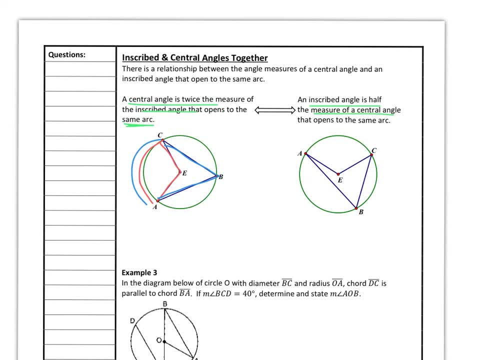 So let me give you an example with this: If I tell you that the arc is 50 degrees, then we know that the central angle is just 50 because it's equal to its arc. But if I go backwards to find the inscribed angle, 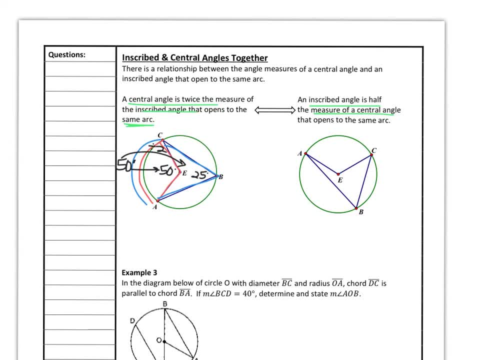 I have to cut it in half, So divide it by 2, and I get 25.. So what we're saying with this phrasing? they mean the same thing. These two are interchangeable. This phrasing says: the central angle measure of angle, CEA. 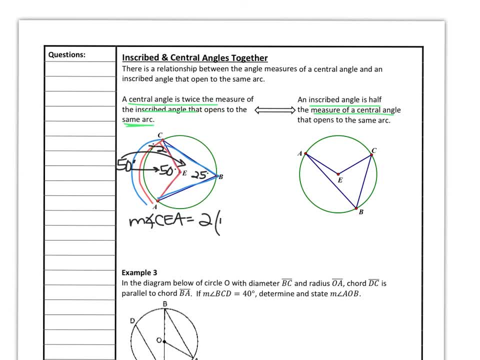 is equal to twice the measure of angle, CBA, the inscribed angle, And that's a true statement, because 50 is equal to twice 25.. Okay, The alternate way of seeing that is again on this picture: central angle opens up to arc AC. 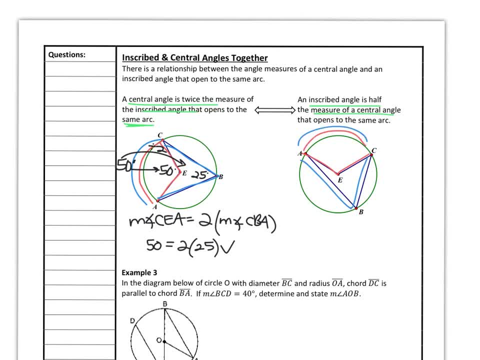 inscribed angle opens up to arc AC. If I tell you again that arc AC is 50, central angle is automatically 50, equal to its arc Inscribed angle divided by 2, and you get 25.. So the opposite way of saying this. 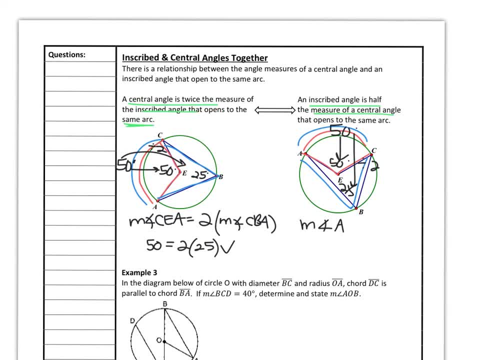 is that the measure of angle ABC or CBA, if you want to call it that way, is equal to half the measure of angle AEC or CEA, if you see it that way. Okay, And again, this is true because 25 equals half of 50.. 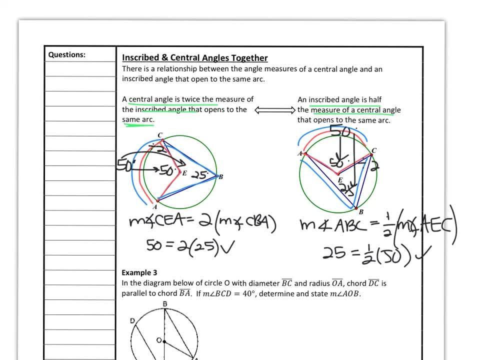 Alright. so you might see a problem where they give you something like this Central angle and then an inscribed angle. They might say: this is 24.. Find out this angle's measure. So you're like, oh, I can do it, I can do it. 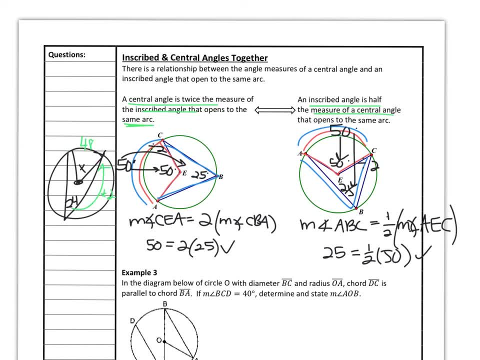 You multiply by 2. That gives you 48 for the arc that they both open up to PS. this would be opened up to it a little bit better And you know that a central angle is just equal to its arc's measure. 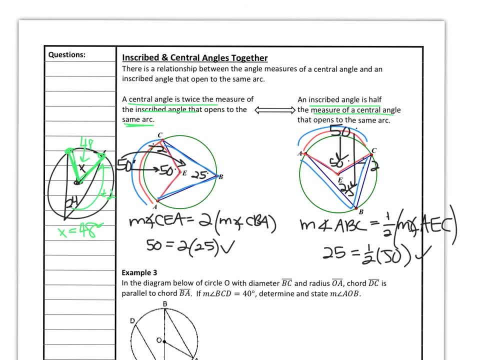 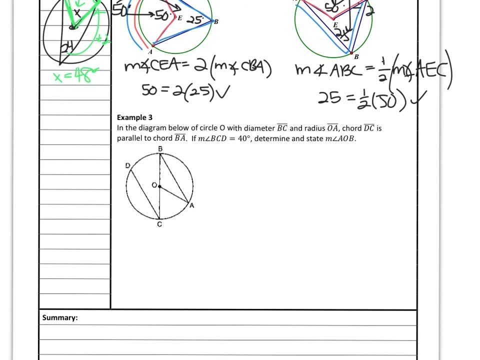 So this is 48.. Okay, Example 3, last and final one. In the diagram below we've got a diameter, a radius and a chord Parallel to DC and BA. Alright, so that's cool As soon as you see parallel lines. 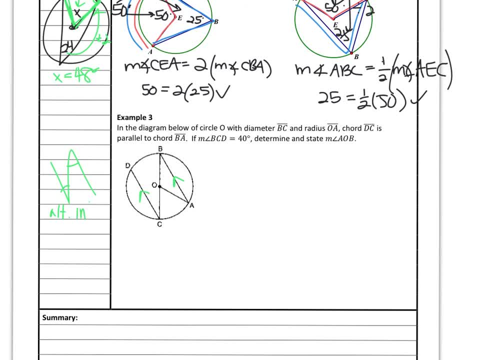 you should be thinking Zs and alternate interior angles. Okay, So if BCD is 40, determine and state the measure of angle AOB. Alright, so I know that this angle is 40. I know alternate interior angles are congruent. 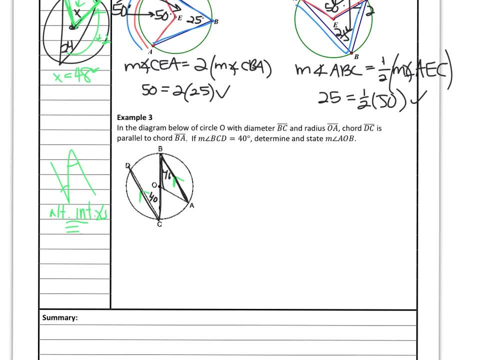 So that means this one must be 40. If you want, we can write out the steps. So step 1 is that measure of angle CBA equals 40. And we'll just write alternate interior. So it's not a problem. 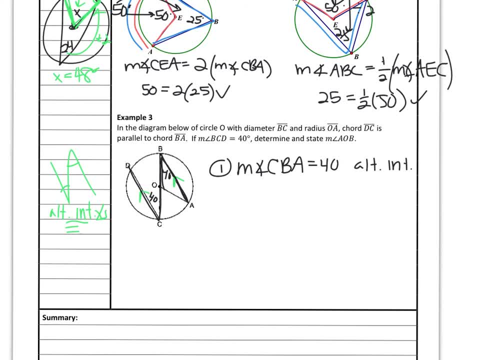 It's not a full explanation because we just have to state the measure, But at least you have the steps to look back at. But then this inscribed angle opens up to arc AC. So if I want to go outwards, I can find the measure of arc AC. 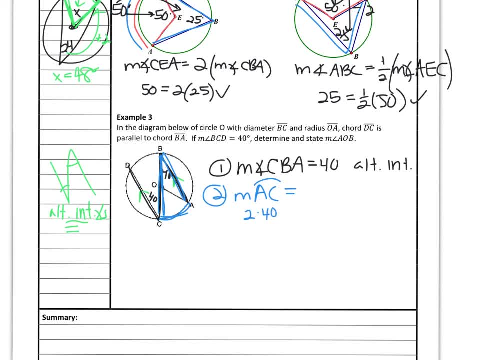 by doing 2 times 40. And that gives me 80.. And that's because inscribed angle equals arc over 2. And then I notice here that I have a diameter, And so therefore arc AB plus arc AC equals 180.. 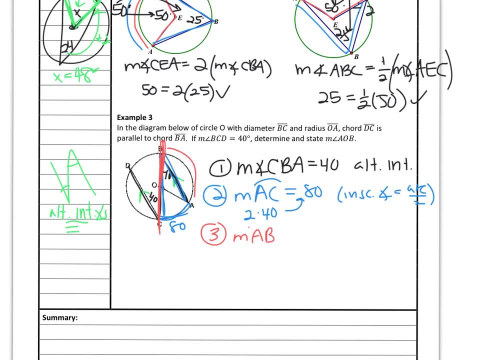 So I can find out arc AB by doing 180 minus 80. And that gives me 100. And that's because a semicircle equals 180.. And then, Oh, let me label that 100.. And then, remember, our goal is to find angle AOB. 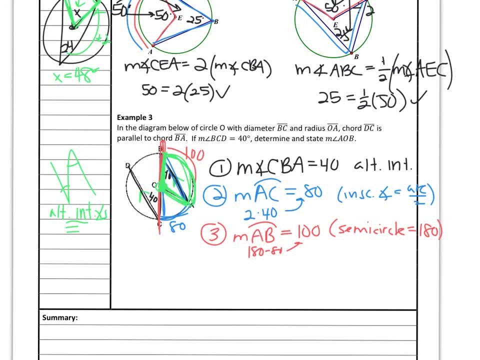 That's a central angle that opens up to arc AB, And so, therefore, if the arc is 100, then measure of angle AOB equals 100 degrees, And that's because a central angle equals its arc. Okay, There are different ways that this could have been done.